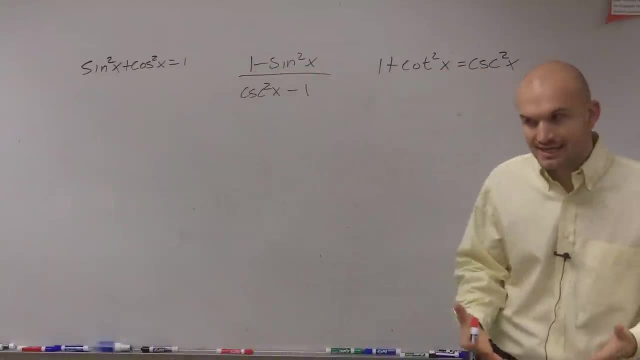 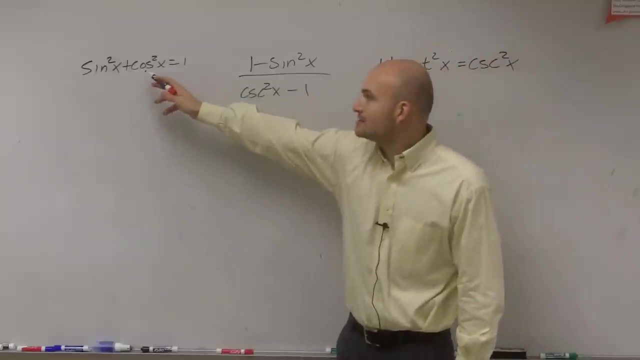 again is: we're going to transform our Pythagorean identities so they can fit into what we're looking for. This says 1 minus sine squared of x. Well, here I have: sine squared of x plus cosine squared of x. So what I showed you guys last time, I don't need to explain. 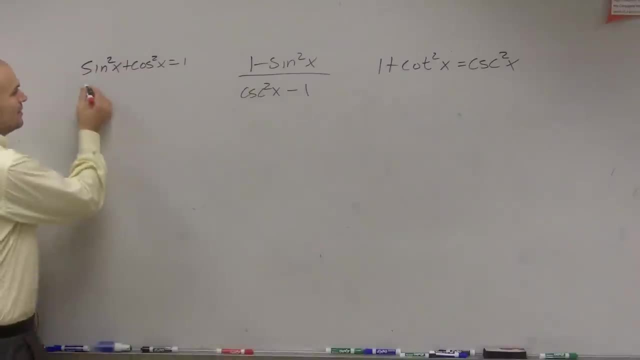 this. I can easily tell you, this, show you guys. this, without talking, is I'm just going to what happens if I subtract sine of x on both sides, Is my equation still going to be the same and equivalent? Yeah, I'm not doing anything, I'm just using the subtraction. 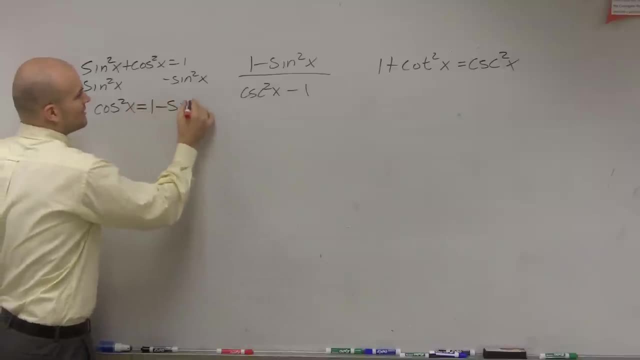 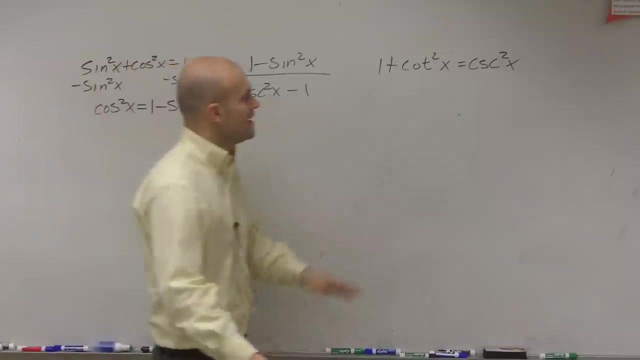 property of equality. So my equation is still going to have the same value, or it's still going to be equal, but now it's just written in a different format, right? All right, Then I can do the same thing here. What about if I just subtracted 1?? I'm not changing the. 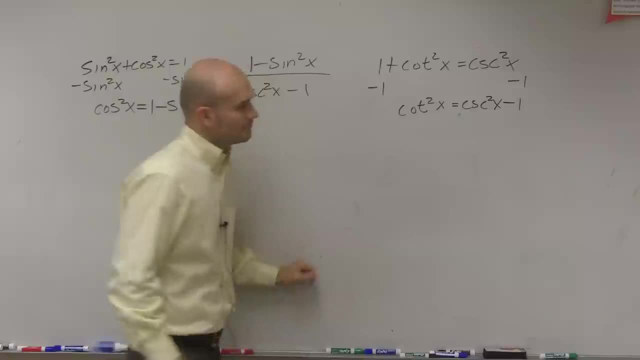 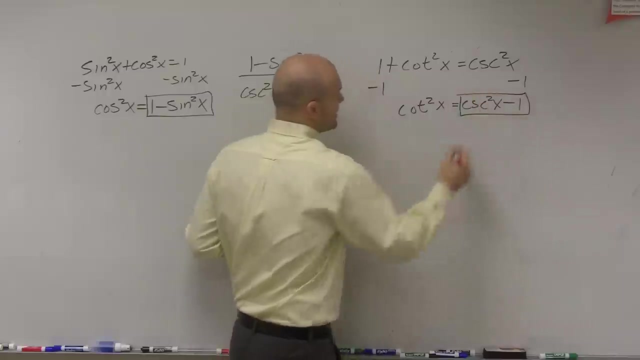 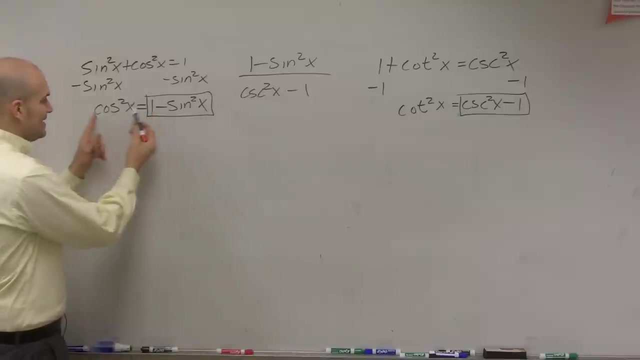 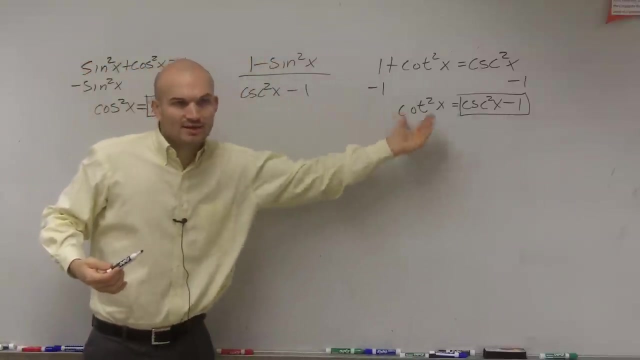 equality of the equation. All right, So now you guys see, I have the numerator right here and the denominator right there, right, But what we want to do is we want to simplify this. So what we say is: since this equals that and since this equals that, how about we put in: we replace what? 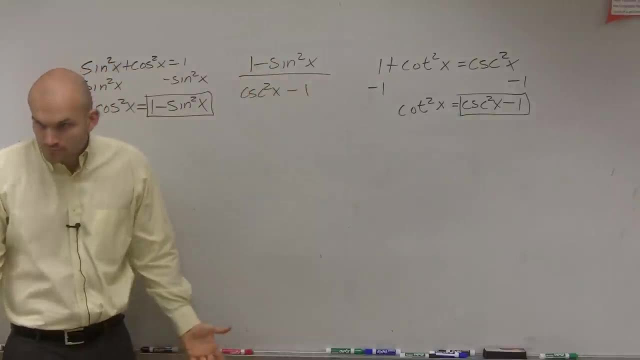 they equal into our function to see if we can simplify it. Does that kind of make a little sense on what I'm doing? All right, So since 1 minus sine squared of x equals, squared of x is equal to cosine squared of x. let's put that up there all over the cotangent. 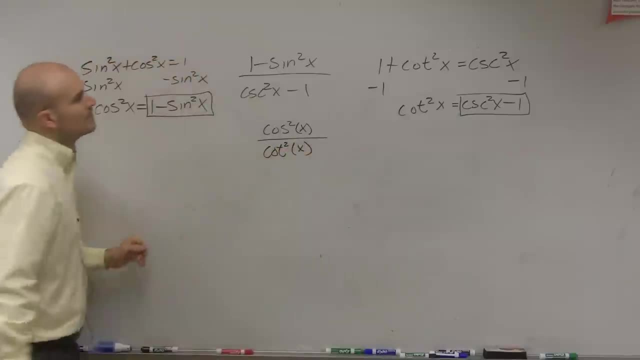 squared of x. okay, So now, so far this looks pretty simplified. This is, you know, simplified down there. but let's see, can we even simplify it even further, all right, So then we look at: well, how about let's try to get rid of a fraction down here. Let's try to get rid of this. 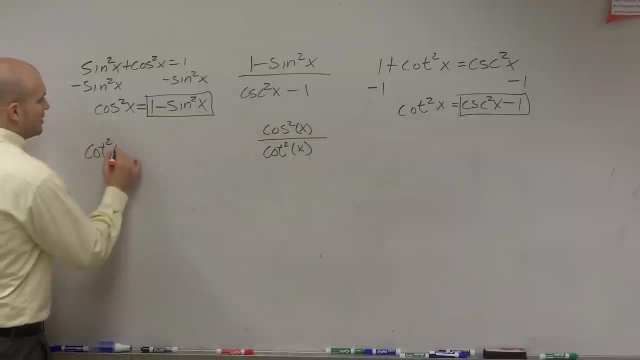 So if we know that cotangent, what is cotangent squared of x going to equal? Well, again, we can apply the quotient identity: The cotangent squared would be the same thing as cosine squared of x divided by sine squared of x, right, Because cotangent is cosine over sine. So if it's squared,